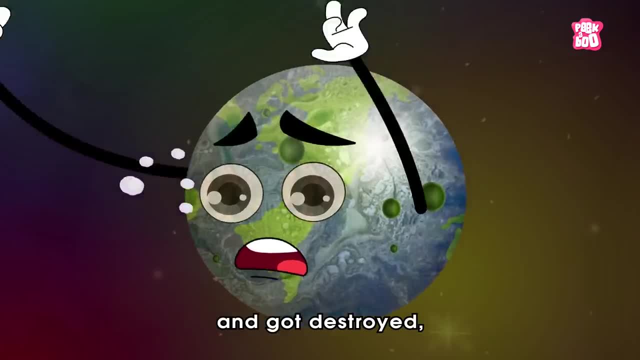 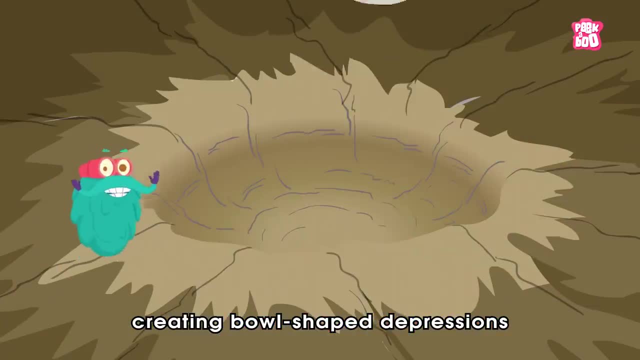 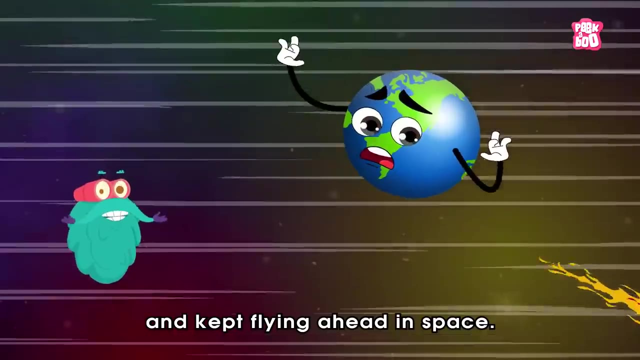 Some of them collided with the earth and got destroyed, While many of them hit the surface, creating bowl shaped depressions called craters, And most of them missed the hit and kept flying ahead in space, Though most traces of the earth's past have long since been destroyed, 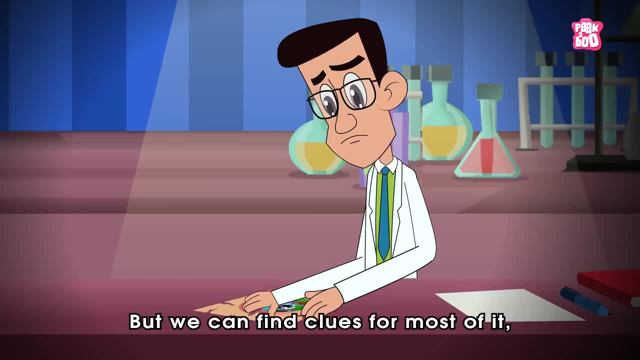 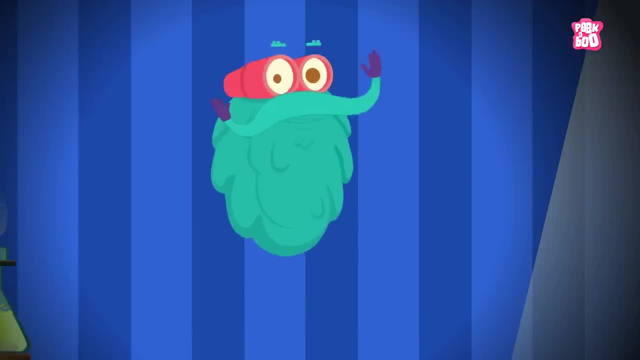 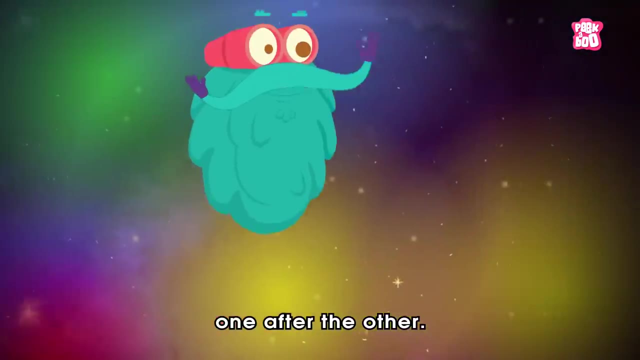 But we can find clues for most of it, And that's why scientists have come up with different theories about space formation, Including the formation of the moon. So let us have a look at them, one after the other. Although there are various theories revolving around the formation of the moon, 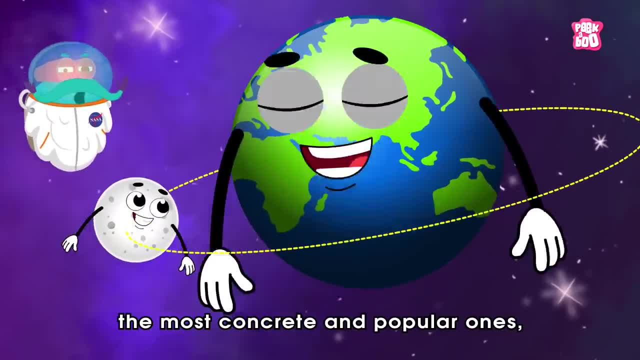 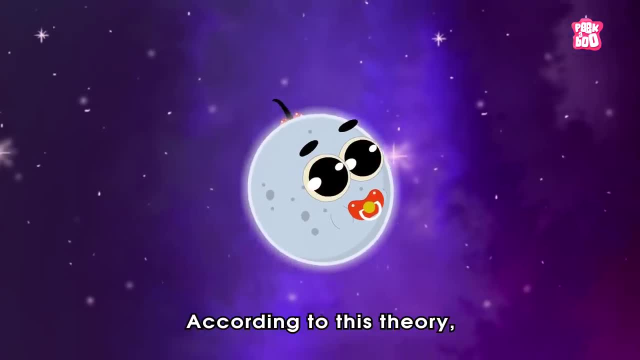 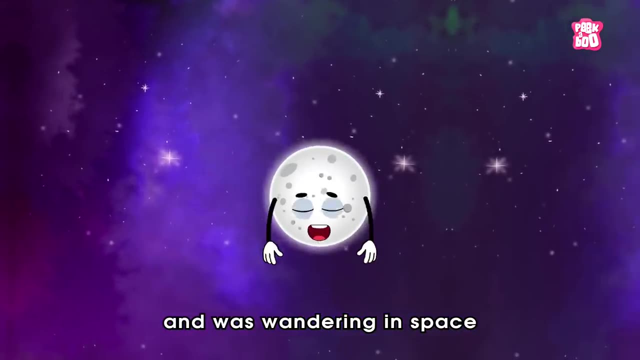 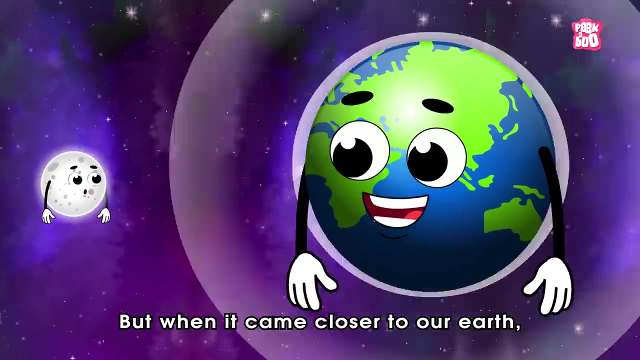 The following. few are the most concrete and popular ones, Starting with the capture theory. According to this theory, the moon was formed elsewhere in the solar system And was wandering in space aimlessly, Unaware of its future, But when it came closer to our earth, it was captured by its gravity. 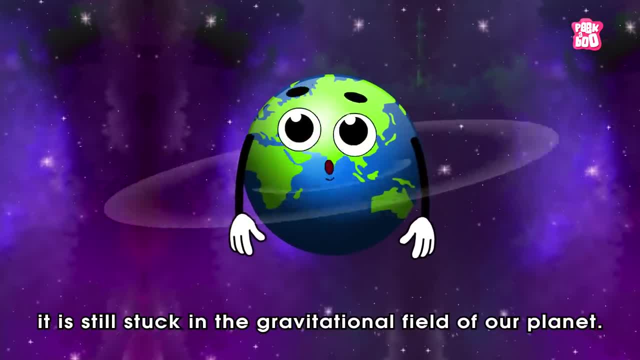 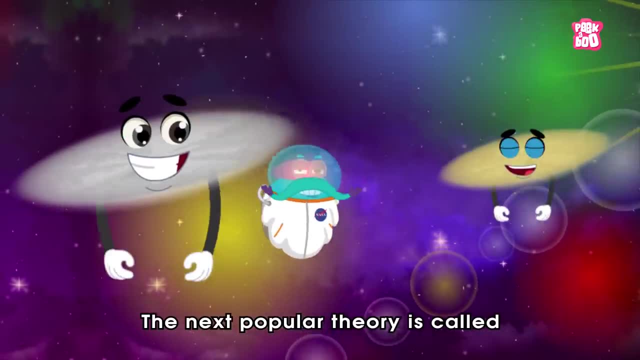 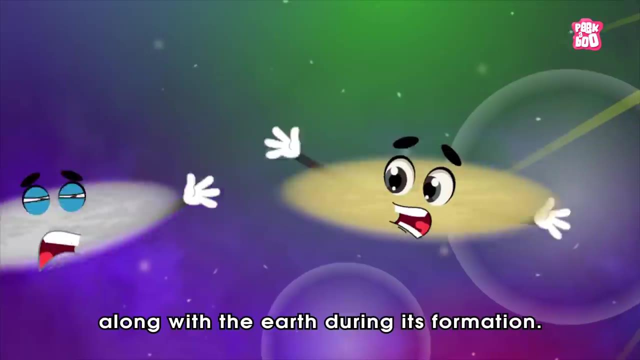 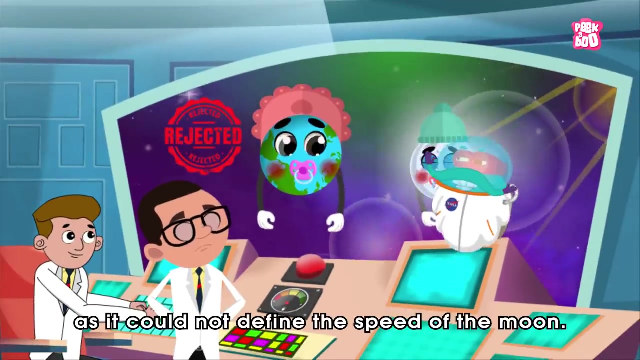 And since it is still stuck in the gravitational field of our planet. The next popular theory is called the accretion theory. This theory suggests that the moon was created along with the earth during its formation. But this notion died out quickly as it could not define the speed of the moon. 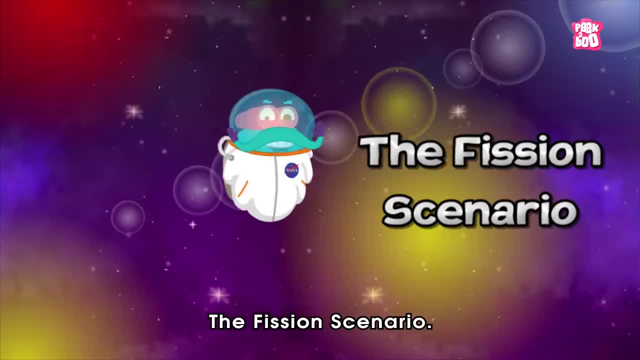 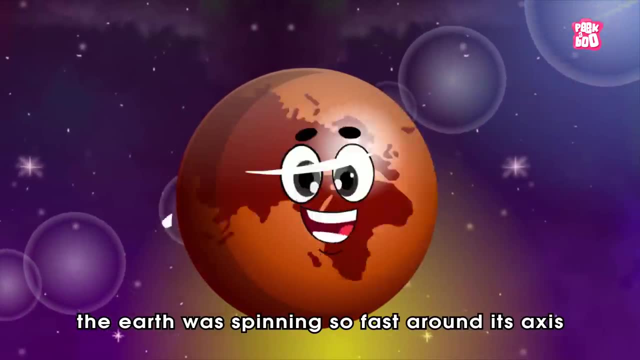 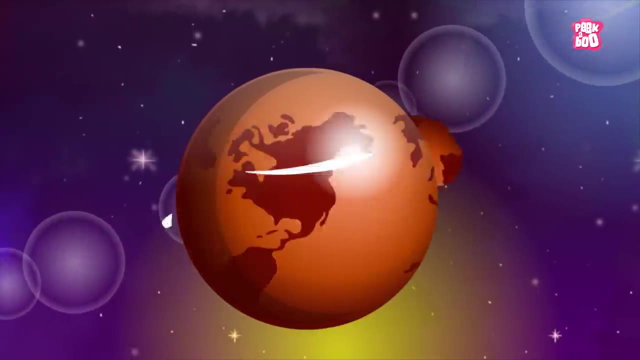 Another popular theory is called the fission scenario. According to this theory, the earth was spinning so fast around its axis That a small part of it broke away and began revolving around the planet. But again, we didn't have much evidence to prove this idea. 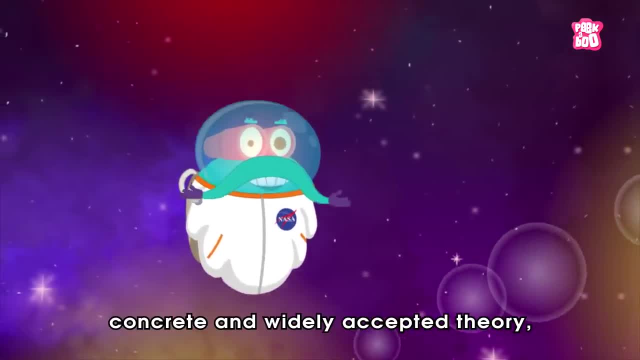 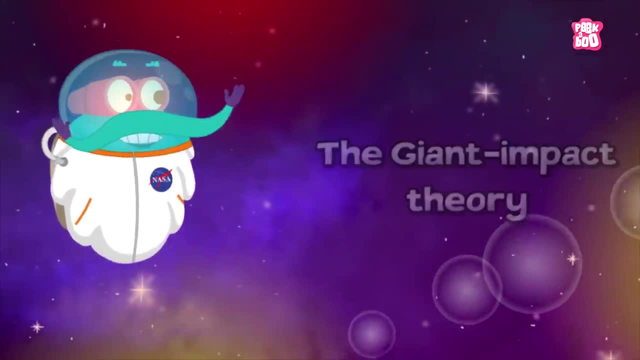 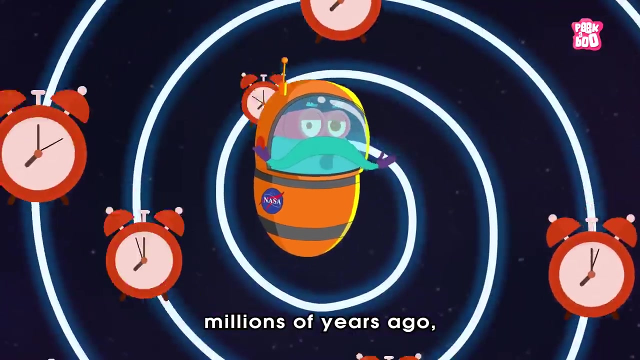 And soon we came up with the most concrete and widely accepted theory, Which is the giant impact theory. Yes, according to the giant impact theory, Millions of years ago, even before the earth and the moon, There existed proto-earth and Theia.